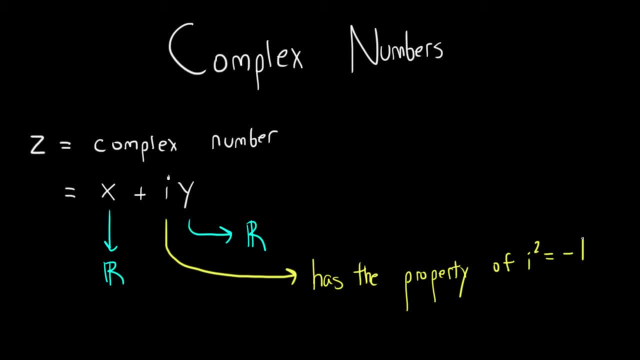 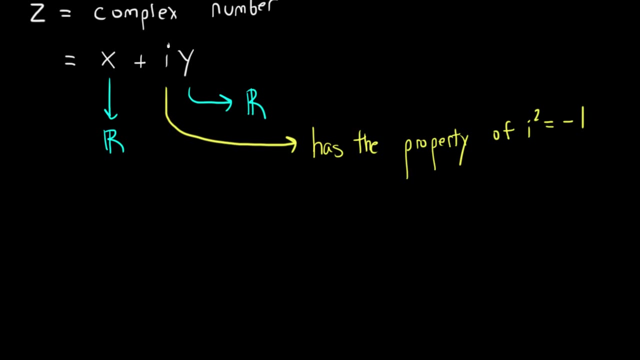 There's going to be more complex numbers than there are real numbers, because we are using real numbers to make this and we are adding another property on top of it. So that's going to allow us to have more complex numbers than we do. So we'll show you one last thing. I'm not going to get this too involved here. I want to keep this video rather basic. 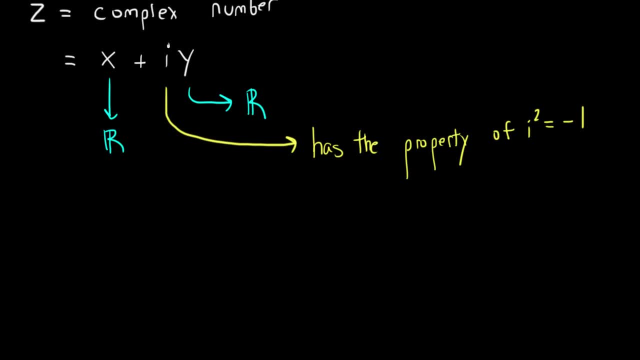 So we're going to, let's go ahead and see how we would write it out. So let's say we want to write out all the complex numbers We are going to. we obviously know that if we use this r over here, this is for real numbers. 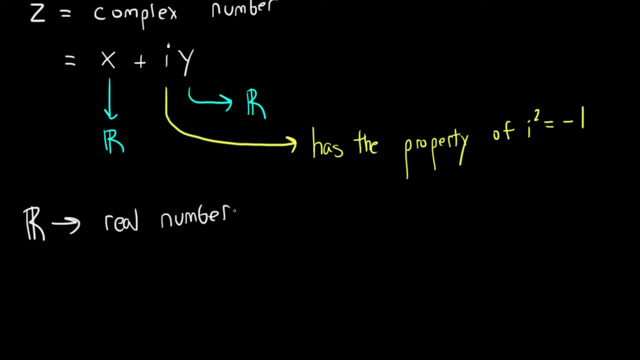 I'm assuming everybody remembers this. So the realm of real numbers is in here, and the one for complex numbers is going to be shown like this: So this is going to be complex numbers And we can actually go ahead and write out what it's going to be. 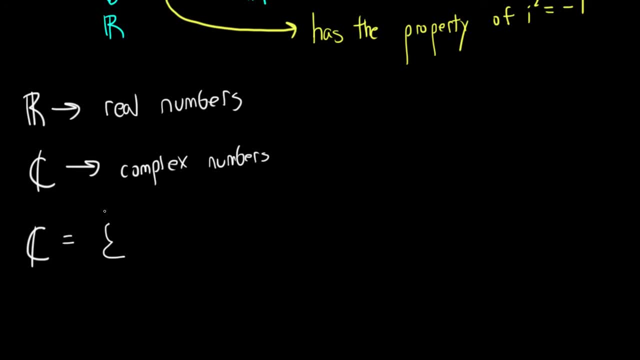 So if we want to write it like this, we can say that the set of complex numbers, it will be x plus i, y, And this obviously you'll have to specify where x and y are part of the realm of real numbers And you don't have to write anything about i. 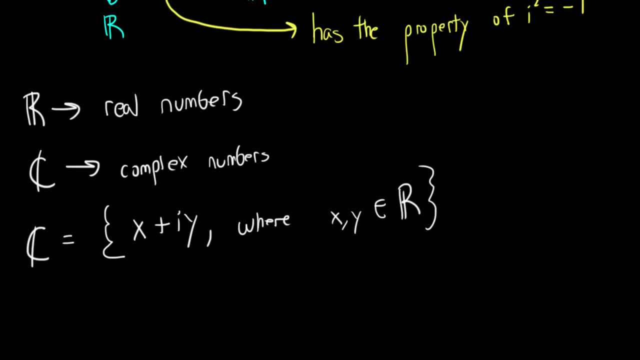 You can just leave it like that And you can go ahead and we can draw this on a little plane if we want to just get a bit more specific, So we can go and we can write this out. So this will be r here. 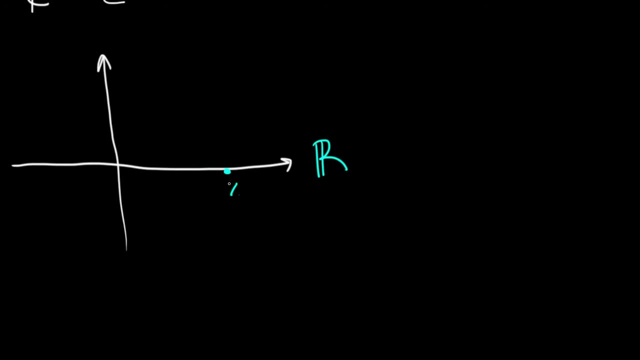 This axis will represent r And we'll have x, We'll have y And these will meet up at some point over here. Go ahead and we can draw some dotted lines to connect them, And this point over here is going to be your x plus i, y. 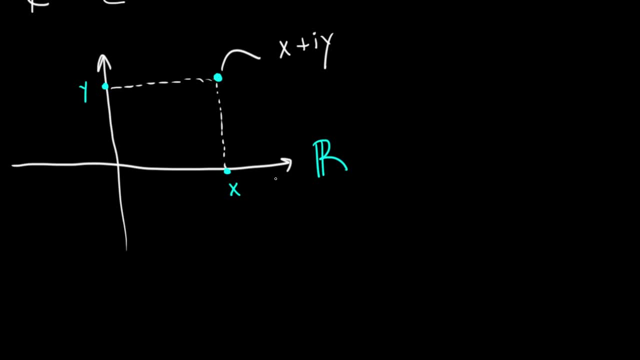 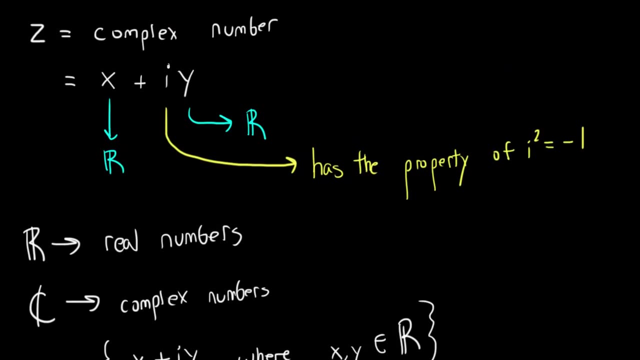 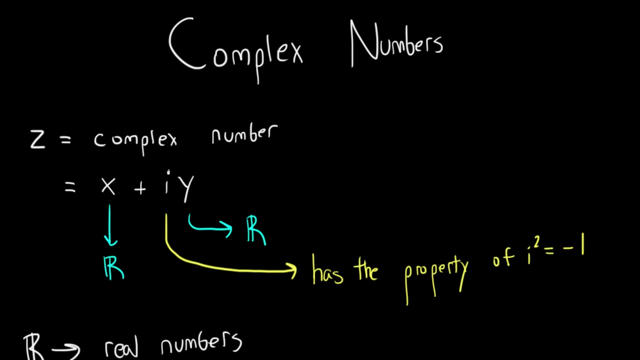 So that's where the point is going to be, And this axis here is representing the real numbers. So let's say, just So that's a brief introduction to complex numbers, We're going to see how we can add them and how we can multiply them in the next video to just get a little bit of a bit more of an understanding about why it's important to have these. 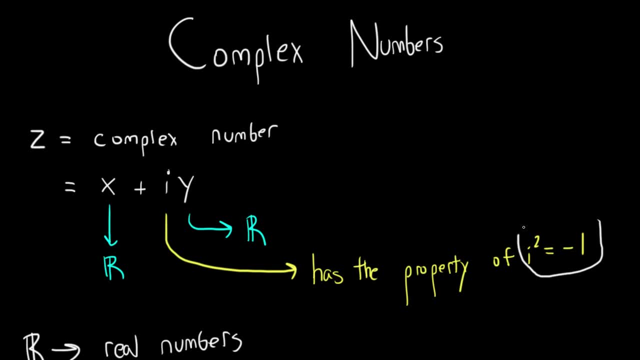 But we need to remember this property of i squared right. This property that i squared is equal to negative one is what makes this so important. So that's essentially the brief overview of complex numbers. You have any questions or you want a bit more detail? leave a comment below and I'll either make a more detailed video or I'll just answer you straight up, if it's an easy question. 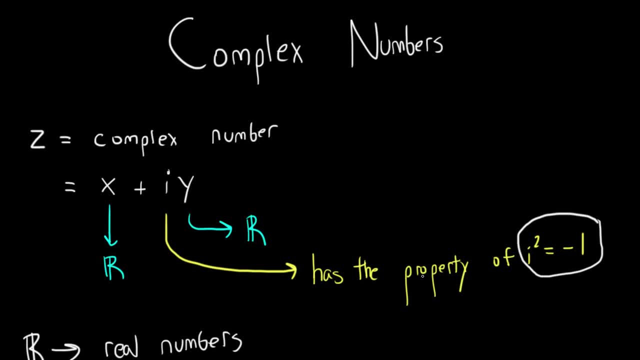 Thanks for watching. If this video helped you, make sure you subscribe. it means a lot and I'll see you in the next video.